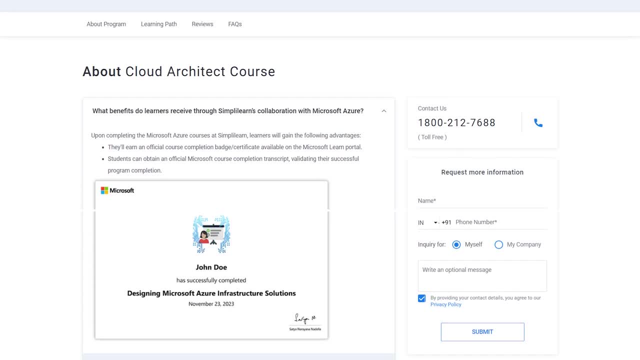 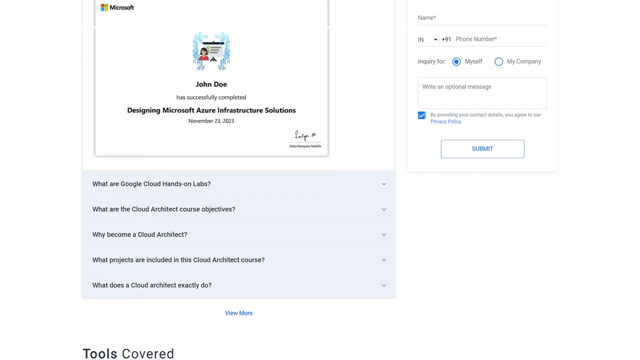 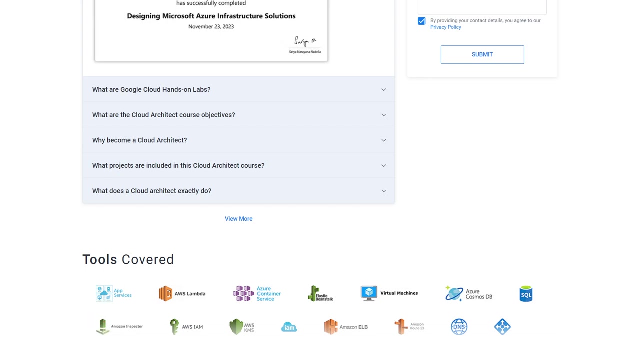 highly scalable and resilient applications, making you job-ready to transform yourself into a proficient cloud professional. And the best part, The program includes an Azure Excel voucher and 100% job assistance from Simply Learn. Check out the course link in the description and pinned comments below. 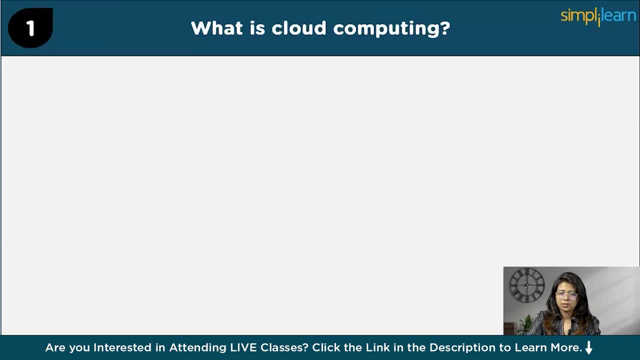 Now let's start with the first question. What is cloud computing? In simple terms, it's like outsourcing your computer needs to a cloud-based cloud platform. It's like outsourcing your computer needs to a cloud-based cloud platform. It's like outsourcing your 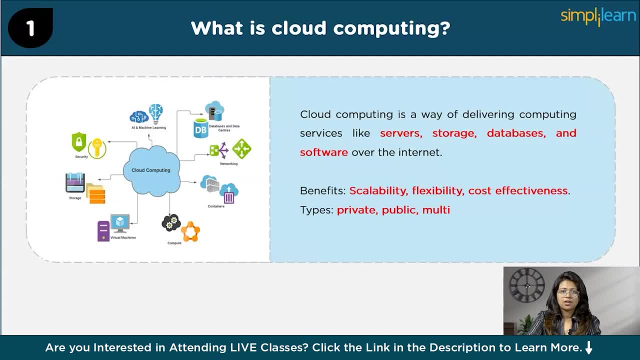 computer needs to a cloud-based cloud platform. It's like outsourcing your computer needs to a remote internet-connected service provider. So you can explain in this way: Cloud computing is a way of delivering computing services like servers, storage databases and software over the internet, Instead of keeping all these resources on your personal computer. 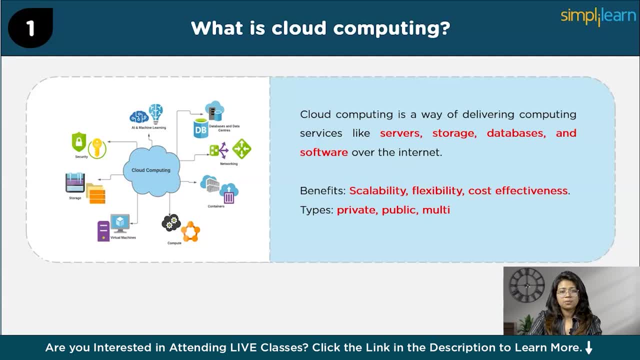 or local server. you access them remotely through the internet. It's like renting computing power and storage space on a massive shared network, which offers benefits like scalability, flexibility and cost effectiveness- cost-effectiveness. We can also talk about different types of cloud computing, like private. 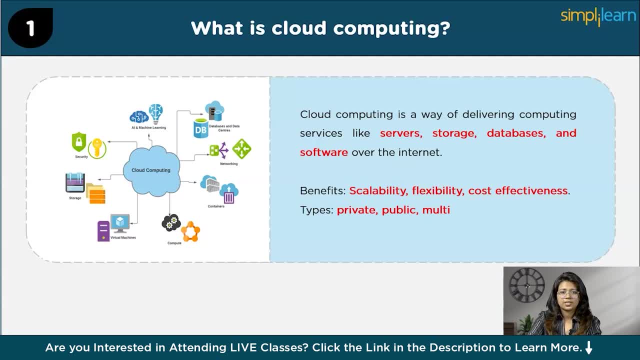 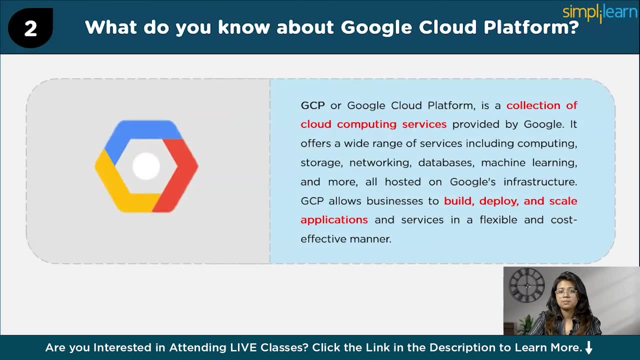 public, hybrid and multi. Now let's move on to the next question: What do you know about Google Cloud Platform? Here it's important to demonstrate your understanding of GCP's key components and its significance. GCP, or Google Cloud Platform, is a collection of cloud computing services. 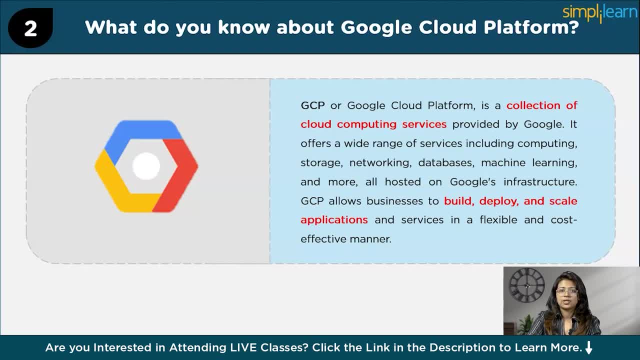 provided by Google. It offers a wide range of services, including computing, storage, networking, databases, machine learning and more, all hosted on Google's infrastructure. GCP allows businesses to build, deploy and scale applications and services in a flexible and cost-effective. 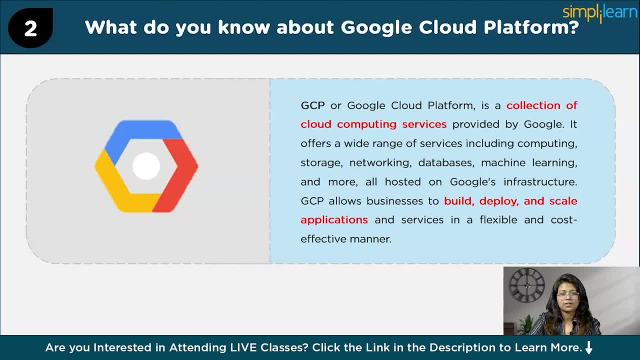 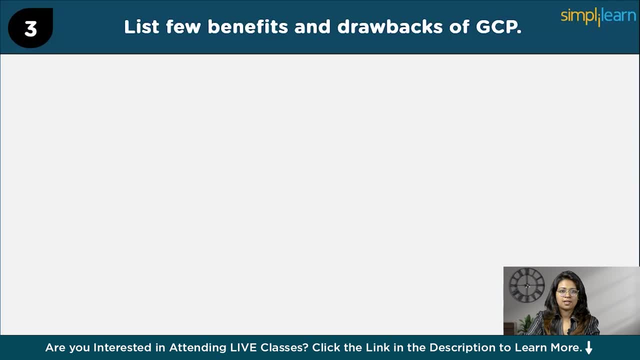 manner. It is widely used by organizations of all sizes across various industries for hosting websites, running applications, analyzing data and developing innovative solutions. Now let's view benefits and drawbacks of GCP In this answer. make sure you provide a balance. 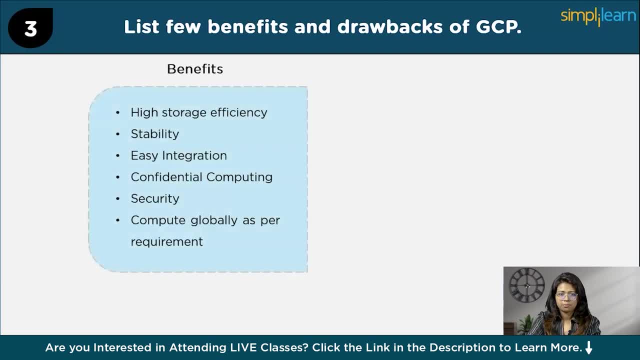 between the benefits and drawbacks of GCP. First, let's talk about the benefits and drawbacks of GCP. Here's how you can approach. Some of the benefits are high storage, efficiency, stability, easy integration, confidential computing, security and compute globally. 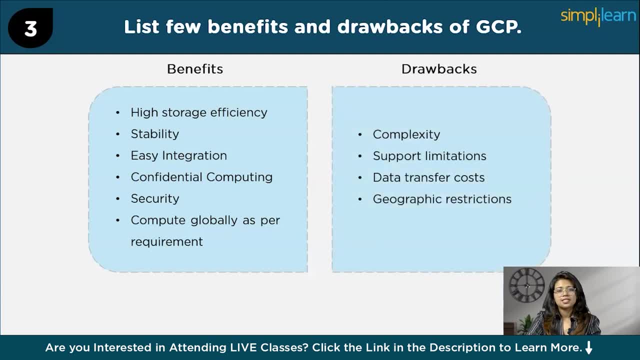 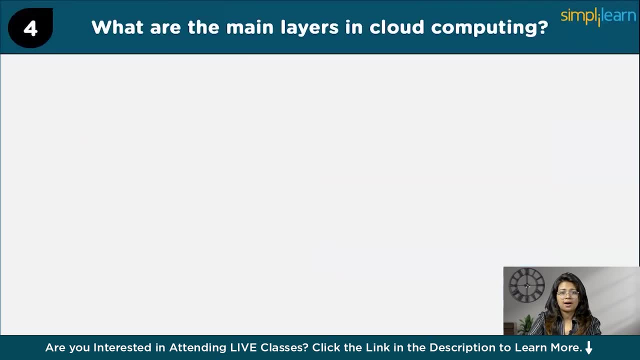 as per requirement. The drawbacks include complexity, support limitations, data transfer costs and geographic restrictions. Now let's see the next question: What are the main layers in cloud computing? You can start by naming the layers first and then briefly describe them. 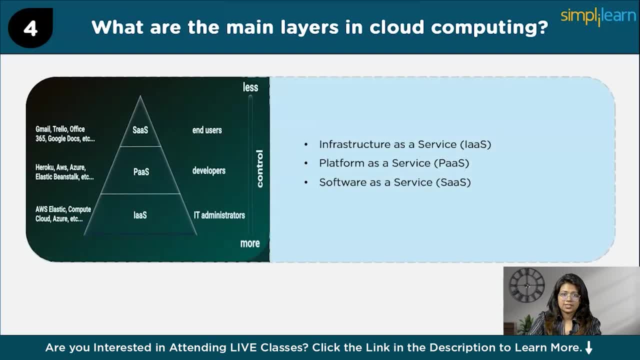 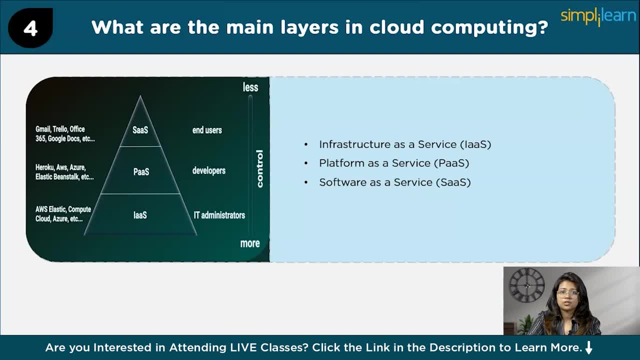 virtualized computing resources over the internet, including virtual machines, storage and networking infrastructure. Examples include AWS, Microsoft Azure, Google Compute Engine, etc. Now, platform as a service offers a platform allowing developers to build, deploy and manage without worrying about underlying infrastructure. 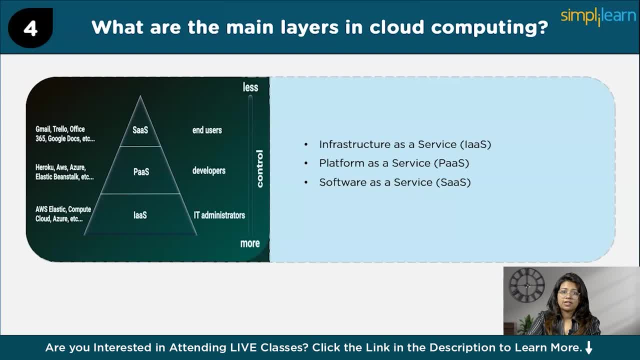 It includes tools and services like databases, development frameworks and application hosting environments. The examples are Google, App Engine, Adopt Commerce, etc. Now comes software as a service, which delivers software applications over the internet on a subscription basis, So users access these applications through a web browser. 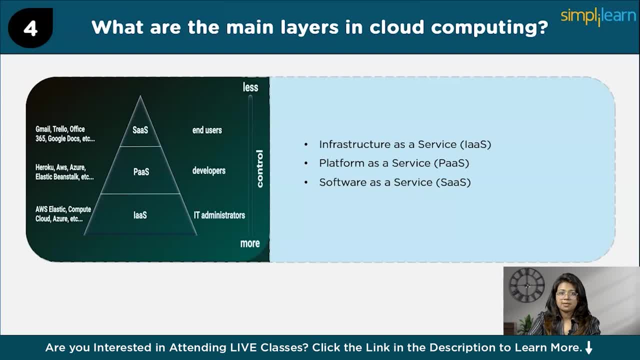 without needing to install or maintain any software locally. Examples include email services, CRM systems and productivity suites like Google Workspace or Microsoft 365.. Now briefly explain the working of GCP. When asked to explain the working of GCP briefly in an interview. 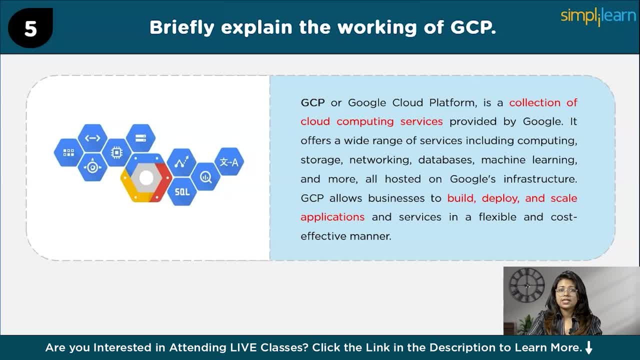 focus on its core principles. So GCP operates by providing a range of cloud computing services over the internet, like storage, computing power, networking, etc. It functions by hosting these services in data centers worldwide and allowing users to access and manage them remotely. 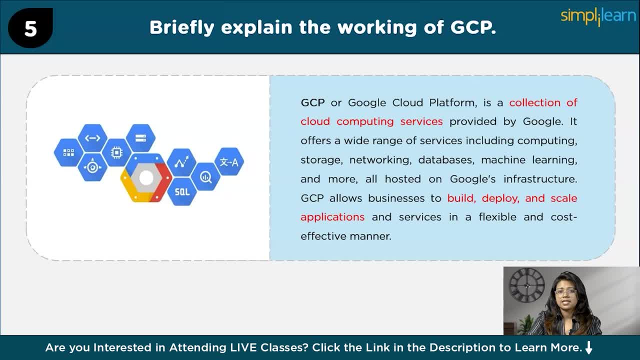 via an internet connection. You can also mention that GCP's infrastructure is designed for scalability, reliability and security, enabling businesses to deploy, manage and scale applications and services efficiently. Additionally, GCP offers various tools and resources for developers, data scientists and IT professionals. 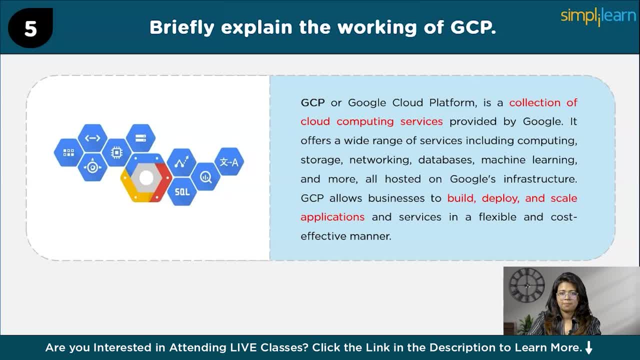 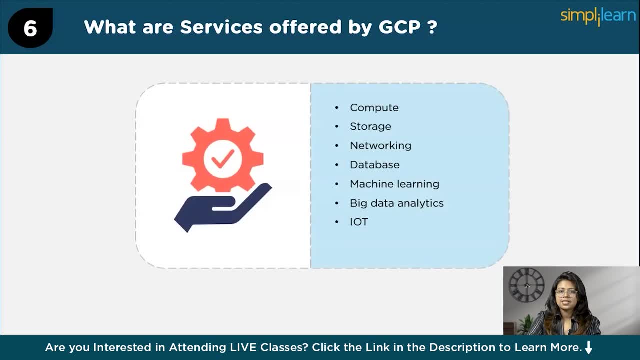 to build, deploy and manage their applications seamlessly. The next question is: what are the services offered by GCP? As already mentioned in some answers, the services include compute storage, networking and databases. You can also highlight specialized services like machine learning. 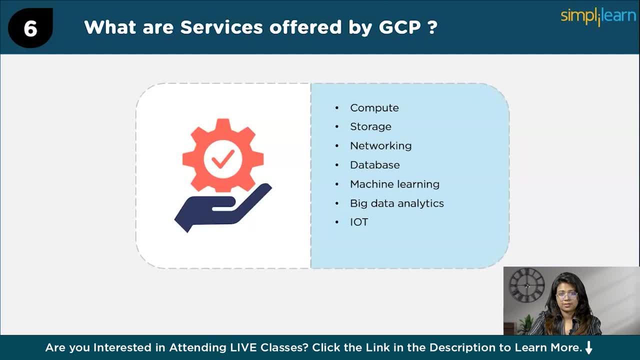 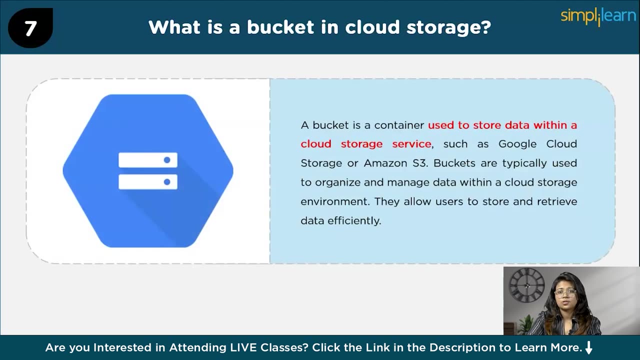 big data analytics and IoT Internet of Things solution. Finally, emphasize GCP's unique features, such as its global network infrastructure and advanced security capabilities. So let's move on to the next question: What is a bucket in cloud storage? So bucket in cloud storage refers to a container. 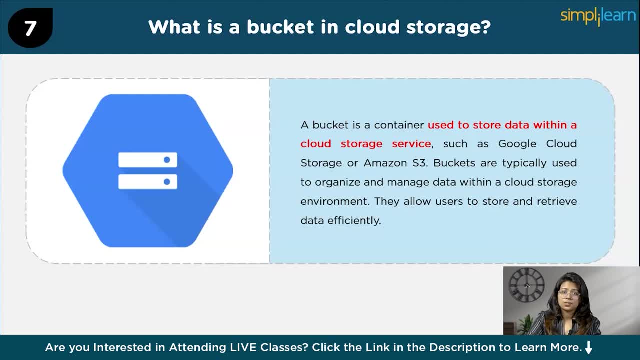 or folder-like structure used to store data within a cloud storage service such as Google Cloud Storage. Think of it as a virtual storage container where you can store files, objects or data. Buckets are typically used to organize and manage data within a cloud storage environment. 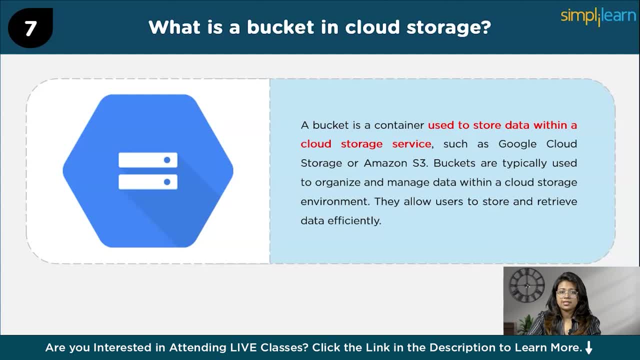 They allow users to store and retrieve data efficiently, and they often come with features for managing access, permissions, versioning and lifecycle policies. Overall buckets play a fundamental role in organizing and managing data within cloud storage system. Now let's see what's the next question. 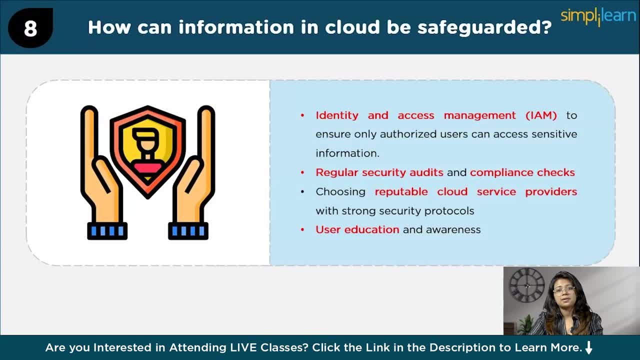 How can information in cloud be safeguarded? So start by highlighting encryption methods to protect data both in transit and at rest. Discuss robust access control measures like Identity and Access Management, IAM, to ensure only authorized users can access sensitive information. Mention regular security audits and compliance checks. 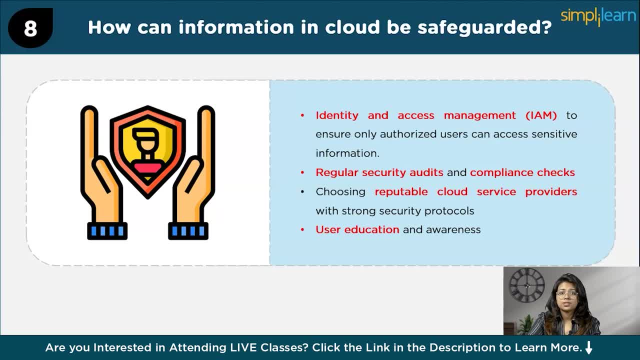 to maintain a secure environment. Emphasize the importance of choosing reputable cloud service providers with strong security protocols in place. Finally, you can mention the significance of user education and awareness, as well as the role of cloud service providers to prevent data breaches due to human error. 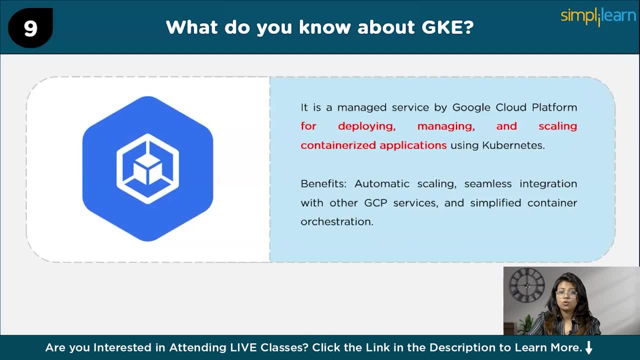 Now, what do you know about GKE? So explain that GKE stands for Google Kubernetes Engine. It is a managed service by Google Cloud Platform for deploying, managing and scaling containerized applications using Kubernetes. Talk about its benefits, such as automatic scaling. 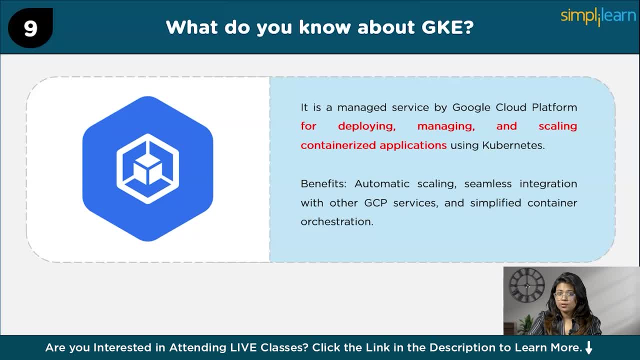 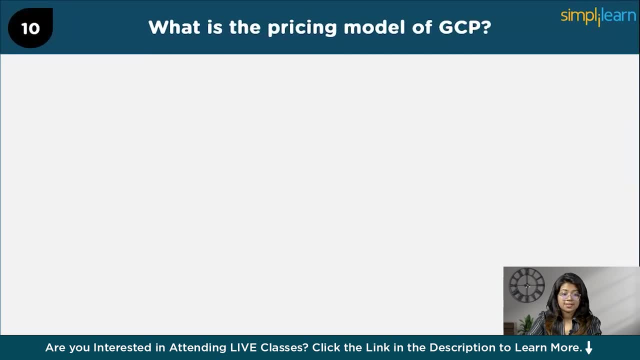 seamless integration with other GCP services and simplified container orchestration, but also highlight your understanding of its role in application development and deployment. The next question they can ask is: what is the pricing model of GCP? So, in answering the question about the pricing model, 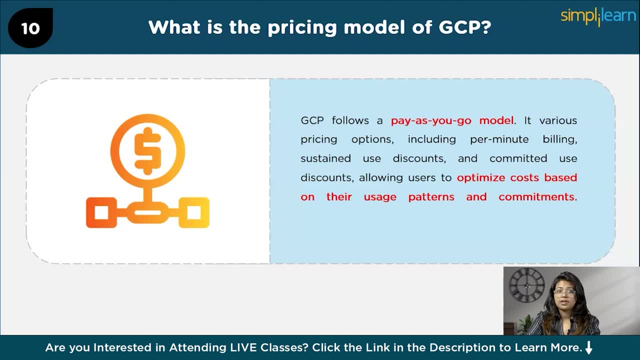 you can explain that GCP follows a pay-as-you-go model, where users are charged only for the resources they consume. Additionally, GCP offers various pricing options, including permanent billing, sustained use discounts and committed use discounts, allowing users to optimize costs. 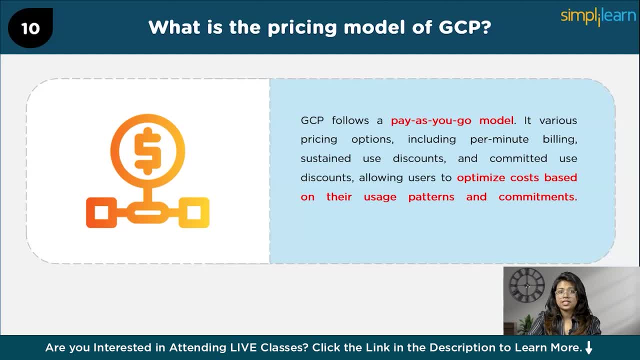 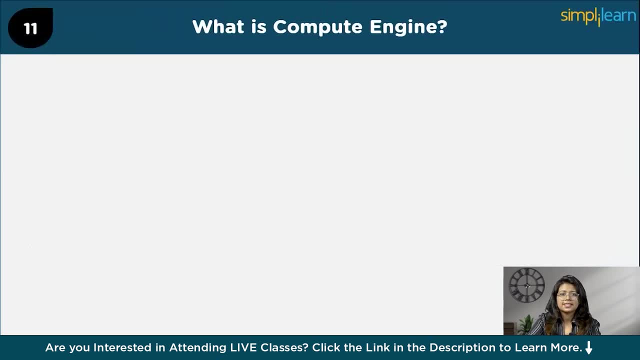 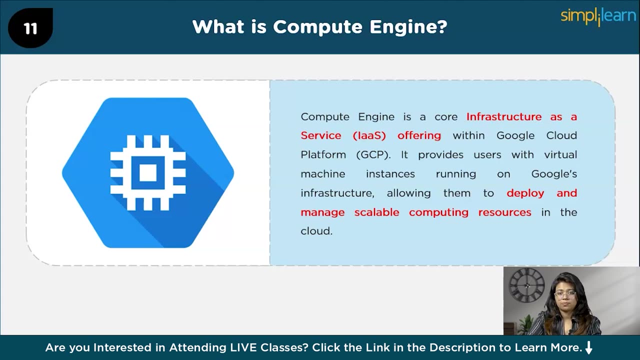 based on their usage patterns and commitments. It's important to highlight GCP's transparent pricing structure and flexibility in accommodating diverse business needs. Now, what is Compute Engine? You can say that Compute Engine is a core infrastructure as a service offering within Google Cloud Platform. 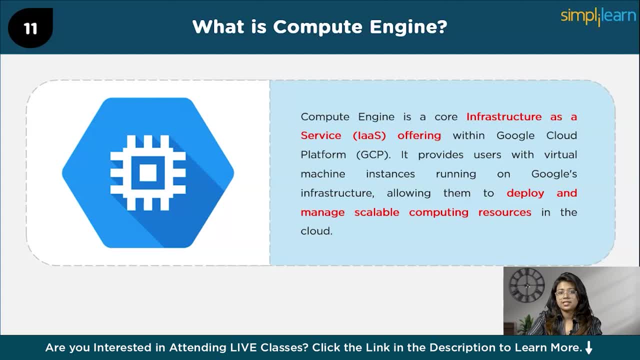 It provides users with virtual machine instances running on Google's infrastructure, allowing them to deploy and manage scalable computing resources in the cloud. So Compute Engine offers flexibility, reliability and high performance for various workloads ranging from small projects to large-scale applications. 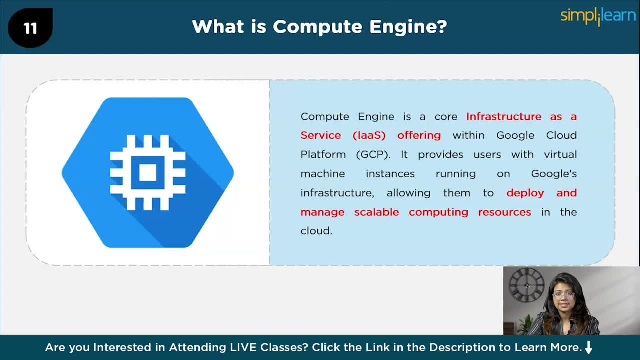 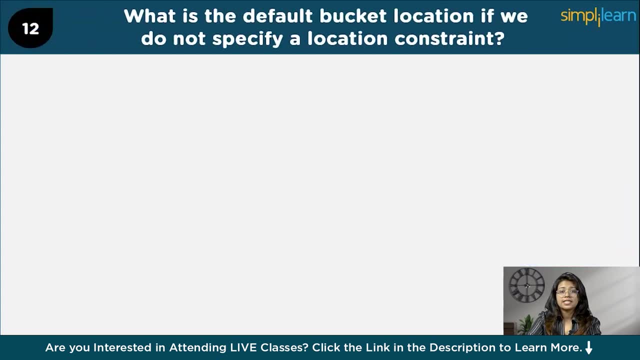 Additionally, you can also mention its integration with other GCP services and the ability to customize instances based on specific requirements. So let's move on to the next question: What is the default bucket location if we do not specify a location constraint? So, when asked about the default bucket location, 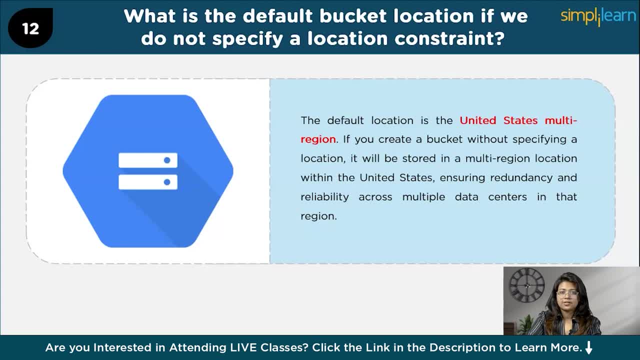 in Google Cloud Storage. if no location constraint is specified, you can respond by stating that the default location is a United States multi-region. This means that if you create a bucket without specifying a location, it'll be stored in a multi-region location. 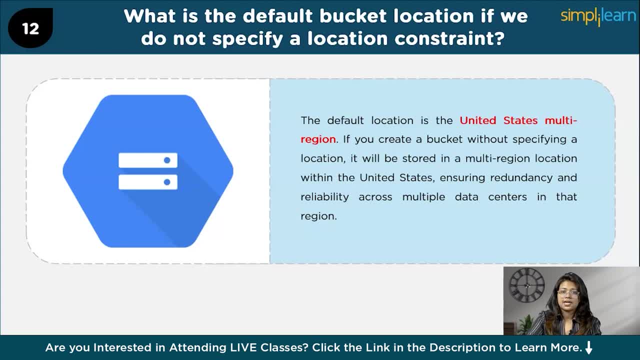 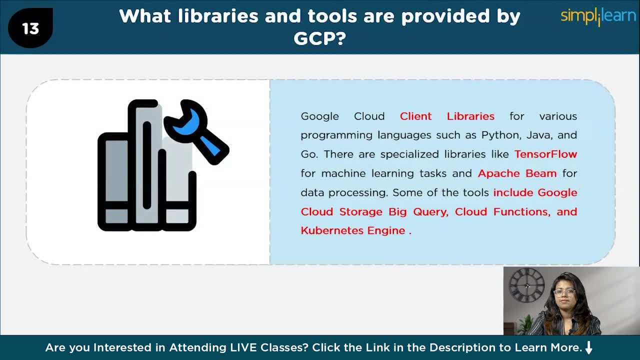 within the United States, ensuring redundancy and reliability across multiple data centers in that region. Now, what libraries and tools are provided by GCP? When addressing this question about libraries and tools, you can mention a variety of libraries and tools available within Google Cloud Platform. 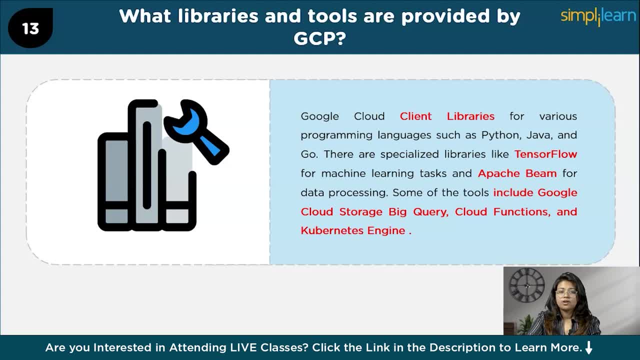 Some notable libraries include Google Cloud Client Libraries for various programming languages such as Python, Java and Go, which provide convenient access to GCP server services. Additionally, there are specialized libraries like TensorFlow for machine learning tasks and Apache Beam for data processing. 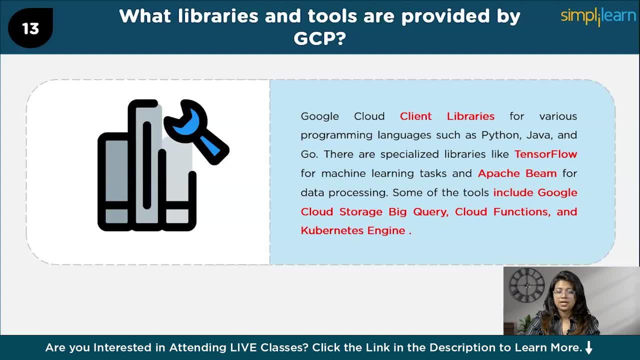 Regarding tools, emphasize widely used ones like Google Cloud Storage for scalable object storage, BigQuery for analytics, Cloud Functions for serverless computing and Kubernetes Engine for container orchestration. By highlighting these libraries and tools, you'll demonstrate familiarity with GCP's robust ecosystem. 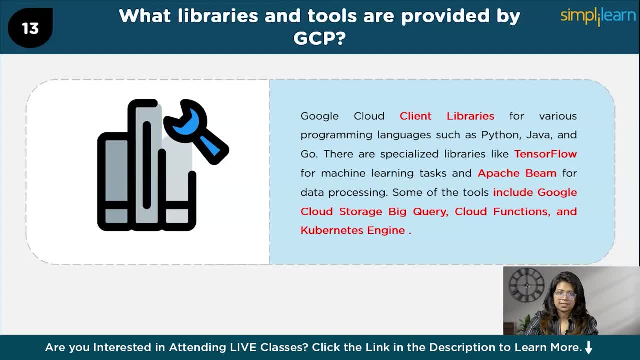 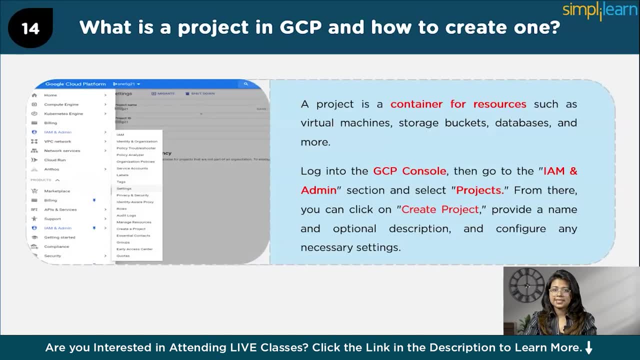 showcasing your readiness to leverage them effectively in your projects or tasks. Now, what is a library? What is a project in GCP, And how to create one? So, in Google Cloud Platform, a project is a container for resources, such as virtual machines, storage. 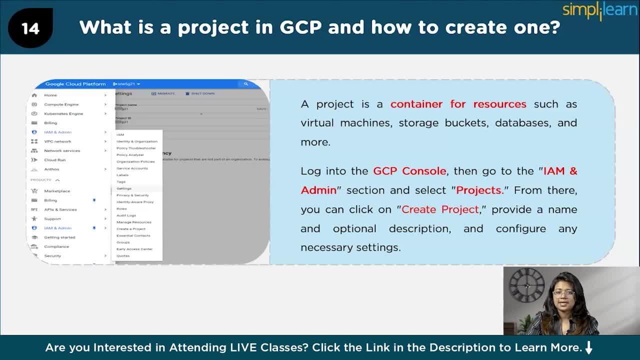 buckets, databases and more, allowing you to organize and manage your cloud services effectively. So to create a program in GCP, you typically start by logging into the GCP console, Then navigate to the IAM and Admin section and select Projects. From there you can click on Create Project. 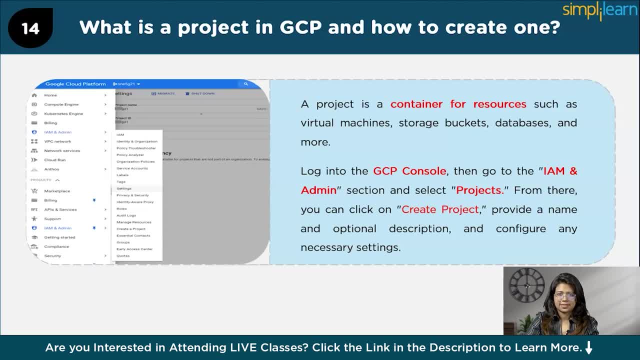 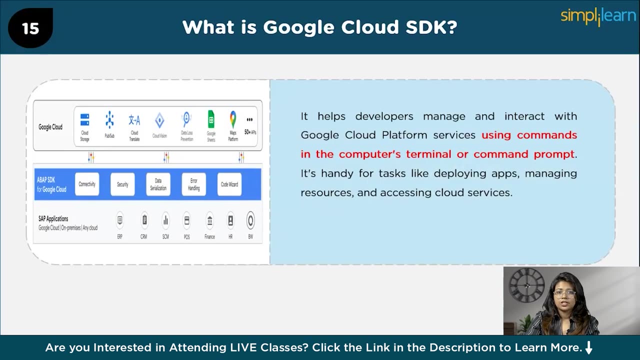 provide a name and optional description and configure any necessary settings. Once created, you can begin provisioning and managing resources within your GCP projects to support your specific use case or application. Now let's move on to the next question, which is: what is Google Cloud SDK? 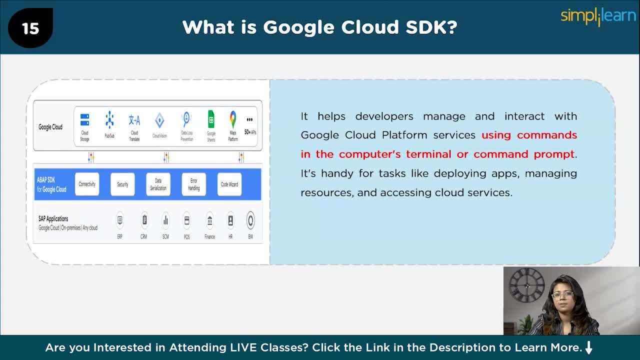 You can say that Google Cloud SDK is like a toolbox provided by Google. It helps developers manage and interact with Google Cloud Platform services using commands in the computer's terminal or command prompt. It's handy for tasks like deploying apps, managing resources and assessing cloud services. 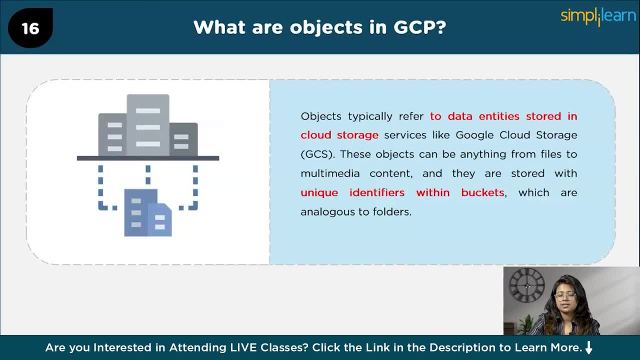 Now, what are objects in GCP? So start by explaining that objects in Google Cloud Platform typically refer to data entities stored in cloud storage services like Google Cloud Storage. So emphasize that these objects can be anything from files to multimedia content, And they are stored with unique identifiers. 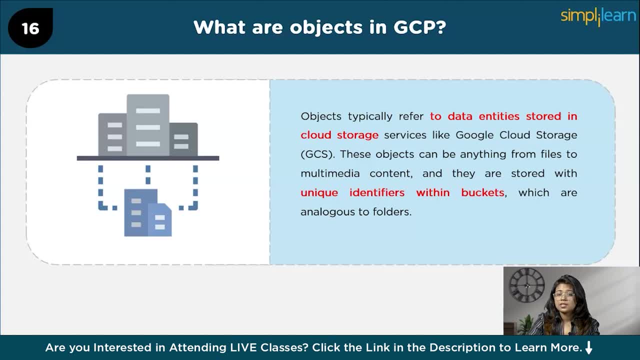 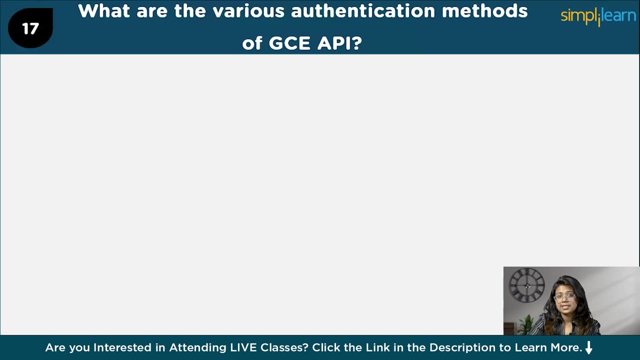 within buckets which are analogous to folders. Also highlight the versatility of objects, as they can be accessed, manipulated and shared across various GCP services, facilitating seamless data management and integration within cloud environments. So what are the various methods for authentication of GCE API? 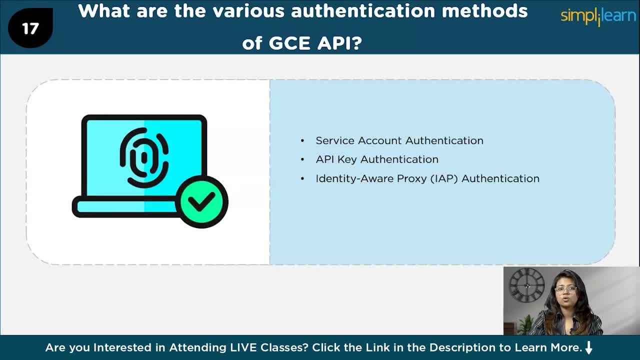 You can mention several methods, after which you can start explaining each, including service account authentication. So this involves creating and using service accounts in Google Cloud Platform to authenticate API requests. So service accounts are associated with projects and can be granted specific permissions. 2.0 authentication. 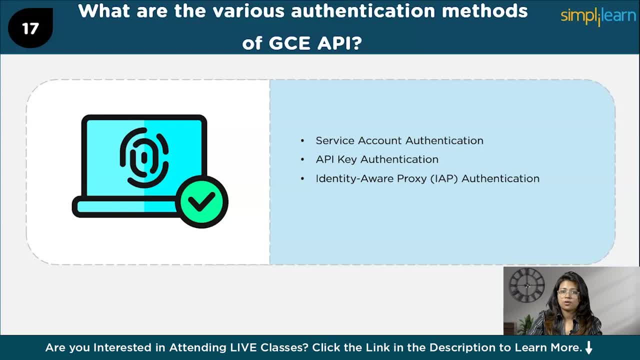 2.0 is a standard protocol used for authorization. GCE API supports 2.0 for authentication, enabling users to obtain access tokens and authentication API requests. The next one is API key authentication. Now, API keys are unique identifiers that developers can generate to authenticate access. 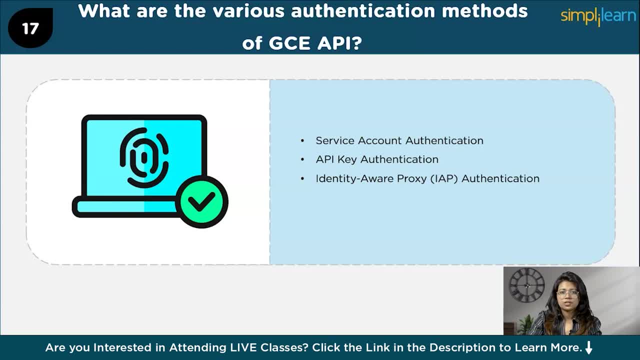 to GCE API endpoints. This method is often used for accessing public data or resources that don't require user-specific permissions. 3.0 Identity-aware proxy authentication. So Google Cloud's identity-aware proxy allows administrators to control access to GCE API endpoints based. 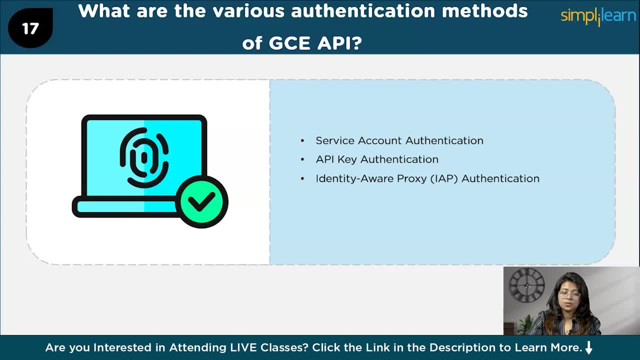 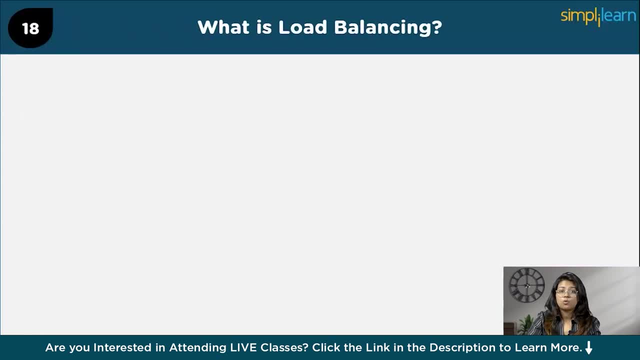 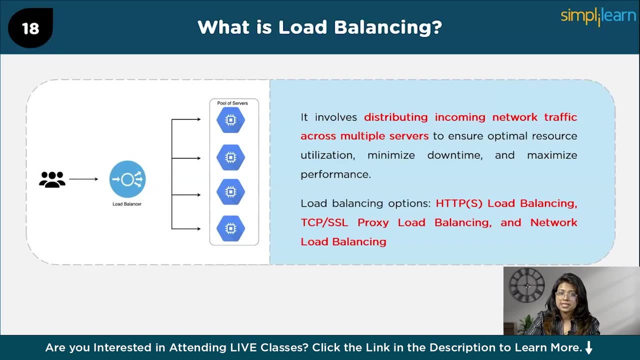 on user identity and context. Users authenticate through Google Identities and IAP verifies these accesses before allowing API requests. Moving on to the next question: what is load balancing? So load balancing in GCP involves distributing incoming network traffic across multiple servers to ensure optimal resource. 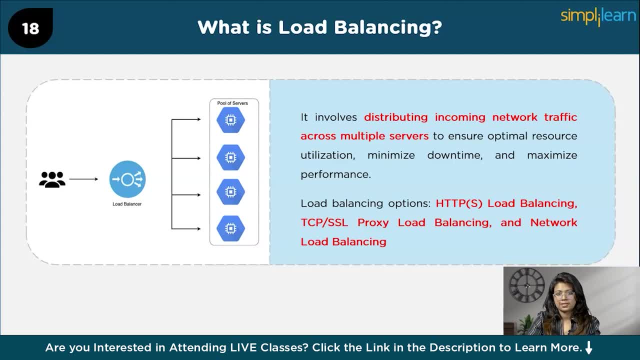 utilization, minimize downtime and maximize performance. Emphasize that GCP's load balancing services automatically adjust to varying levels of traffic, helping to maintain stability and reliability for application and services hosted on GCP infrastructure. You can also mention that GCP offers various load balancing. 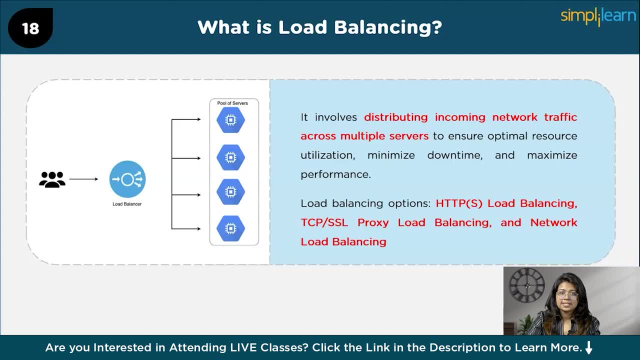 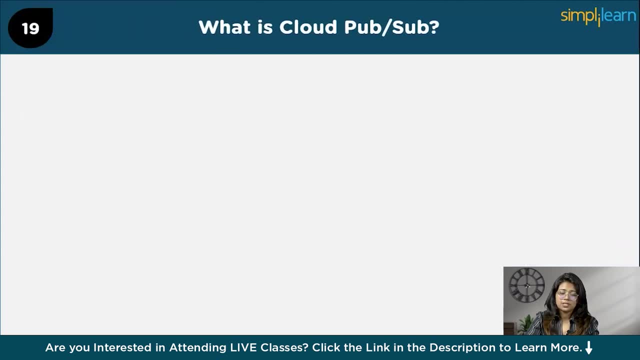 options including HTTPS load balancing, TCP, SSL, proxy load balancing and network load balancing, each tailored to specific use cases and requirements. Now coming to the next question, Let's move on To the next question. what is Cloud PubSub? 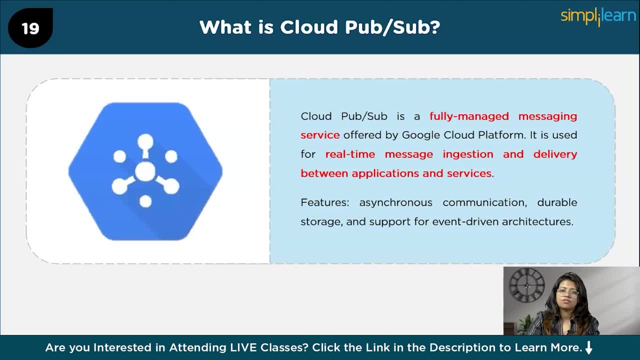 So Cloud PubSub is a fully managed messaging service offered by Google Cloud Platform. You can describe its functionality as a scalable and reliable system for real-time message ingestion and delivery between applications and services. Highlight its key features, such as asynchronous communication, durable storage and support for event-driven architecture. 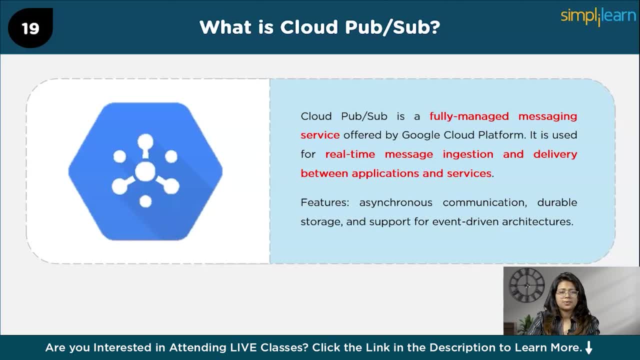 It can emphasize its role in enabling decoupled, scalable and resilient cloud-native applications. Finally, mention its benefits in terms of flexibility, scalability and ease of integration with other GCP services. Now, coming to our last question: what is Google BigQuery? 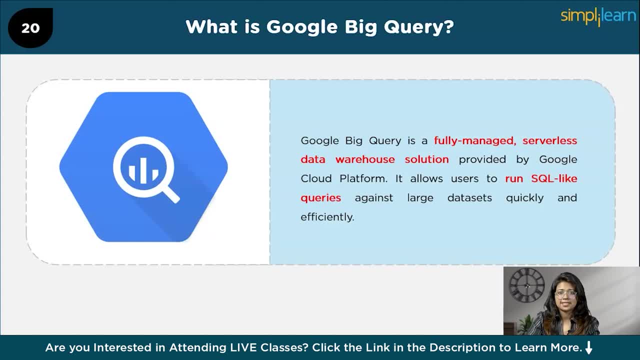 So Google BigQuery is a fully managed, serverless data warehouse solution provided by Google Cloud Platform. It allows users to run SQL-like queries against large data sets quickly and efficiently. Emphasize its scalability, real-time analytics capabilities and seamless integration with other. 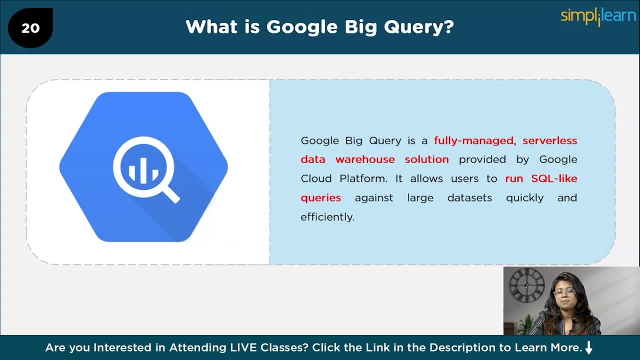 Google Cloud services. And there you are with top 20 GCP interview questions that you can definitely expect in your interview. We have given an overview of each of the topics, But make sure, while you answer the questions during an interview, try explaining the concepts. 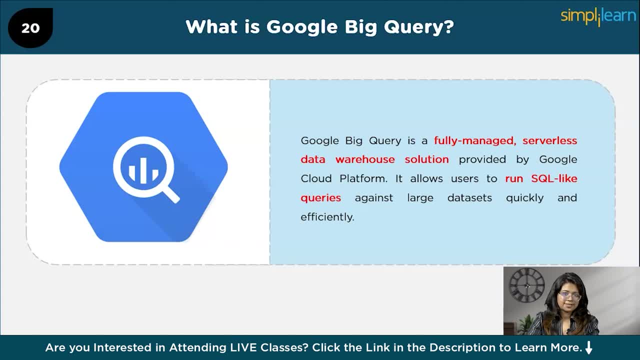 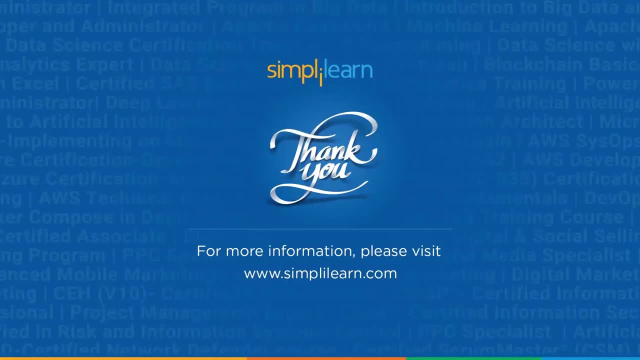 in your own words, so that you can portray your communication skills. Also, mention real-time examples according to your experience. So I hope you found this video informative. If you like this video, do not forget to subscribe and give us a thumbs up. 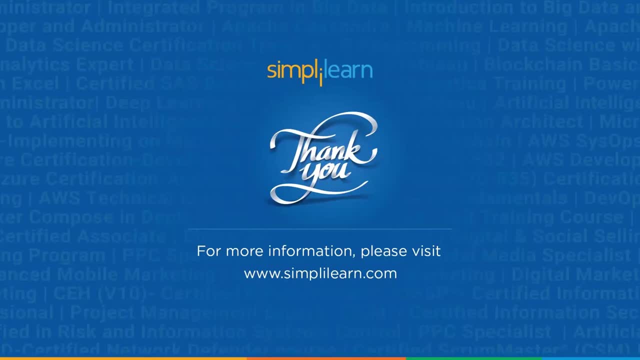 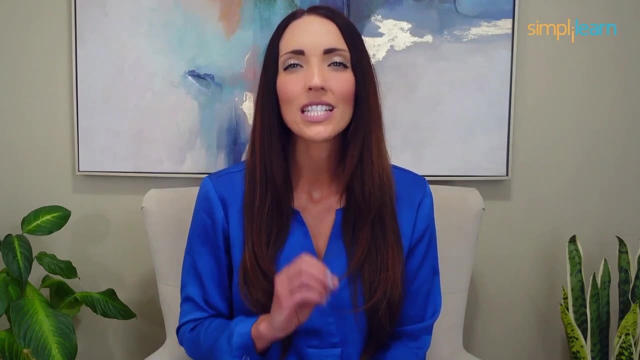 Also check out other videos on this topic from our channel for your preparations. Thanks for watching and we wish you the best of luck for your interviews. Staying ahead in your career requires continuous learning and upskilling, Whether you're a student aiming to learn today's top skills.